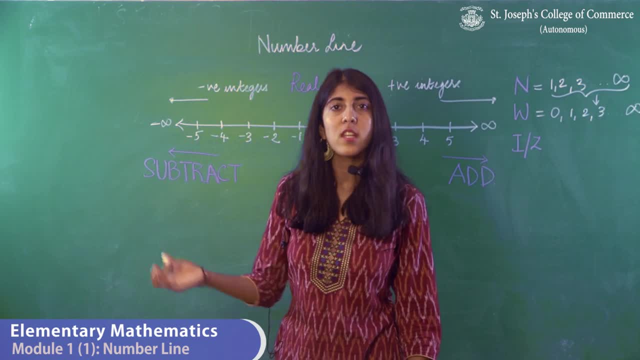 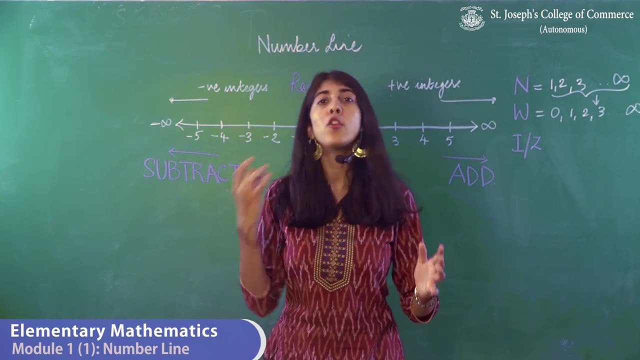 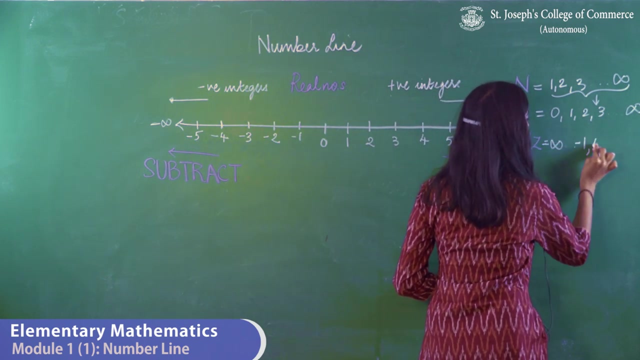 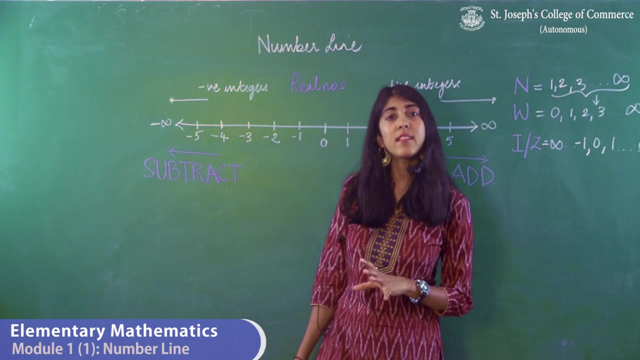 and they move on to minus infinity. Positive integers are one, two, three and they move on to positive infinity. Zero is in the middle and it's neither positive nor negative, But integers are mostly zero, one and they move on to positive infinity. These are integers, The next thing we are. 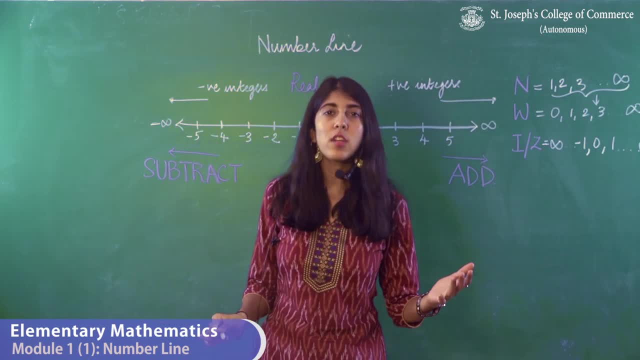 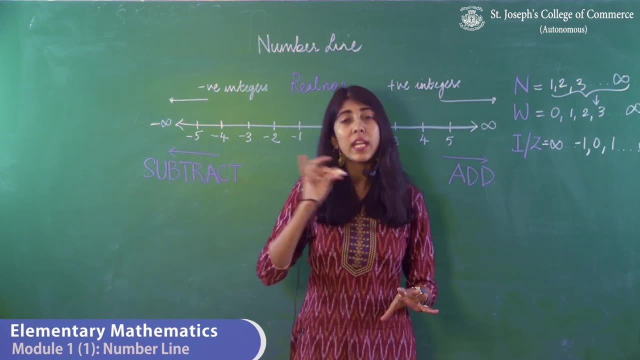 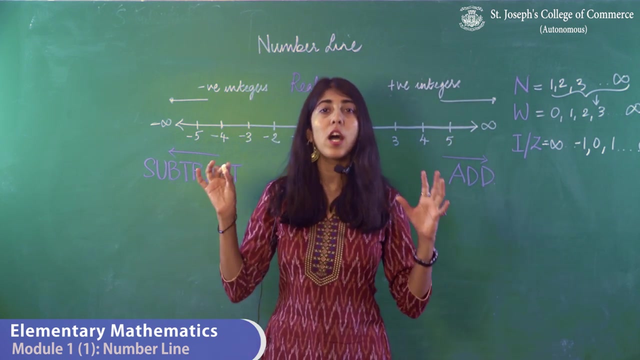 going to look at are rational and irrational numbers. Rational numbers are numbers that can be represented in a ratio or a fraction form, And irrational numbers are any kind of numbers that cannot be expressed. So real numbers are just a combination of rational and irrational numbers. Now the number. 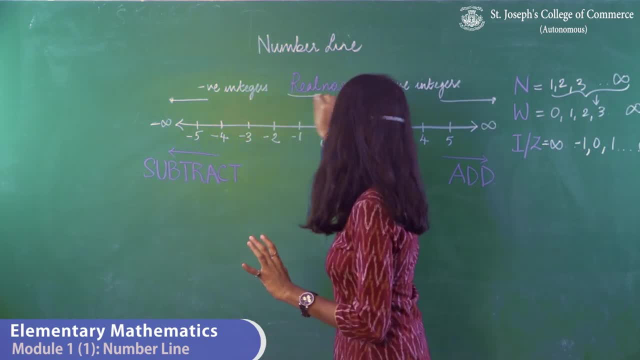 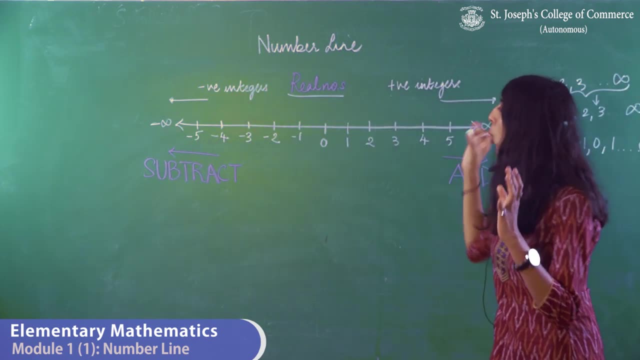 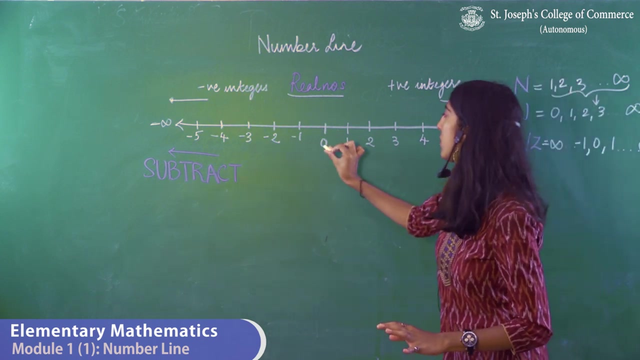 line represents only real numbers. If you have noticed, I have represented the number line and I have written only real numbers here. That means a number line can only accommodate rational and irrational numbers. Moving on to how the number line is represented, If you notice, zero is in the middle to. what does that represent? I have written zero. 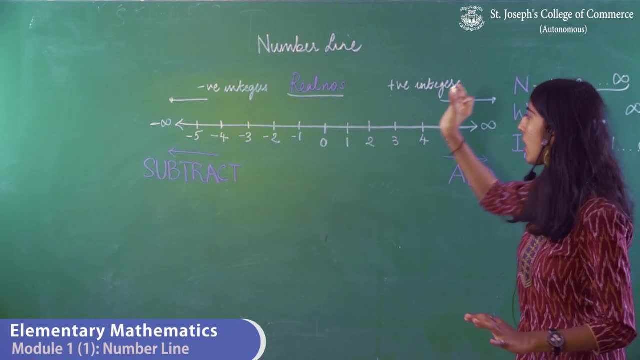 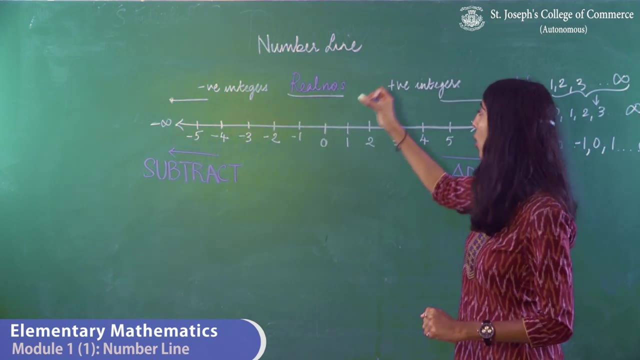 I had written zero before I had written negative and negative Is 0, the same number. I showed the right hand side: you have all positive integers, and towards the left hand side you have all negative integers. When you are solving, you need to know that if you are moving along. 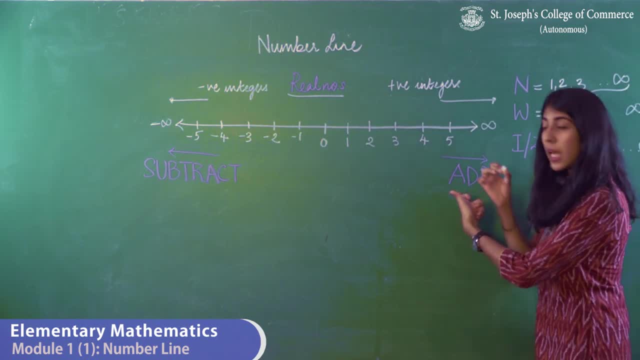 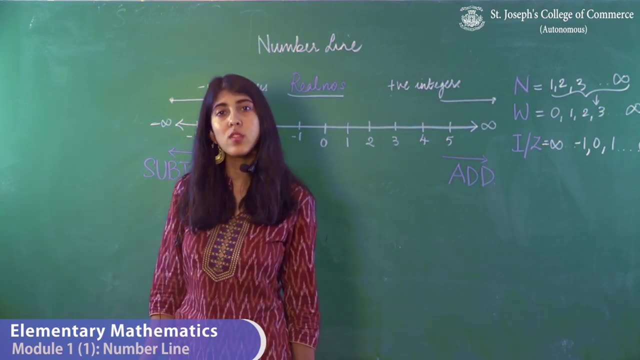 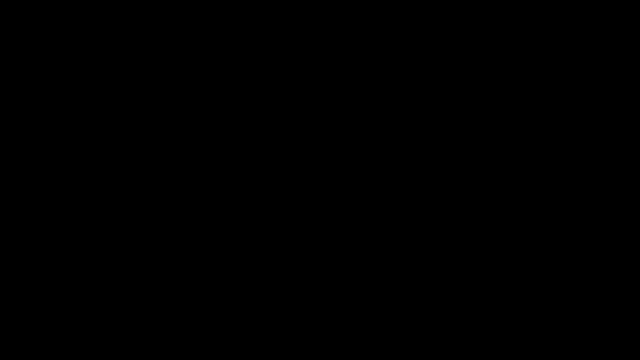 the number line towards the right hand side, you need to add, and if you are moving along the number line towards the left hand side, you need to subtract. Let's move on to understanding the rules required in order to solve the number line. When we need to solve numbers on the 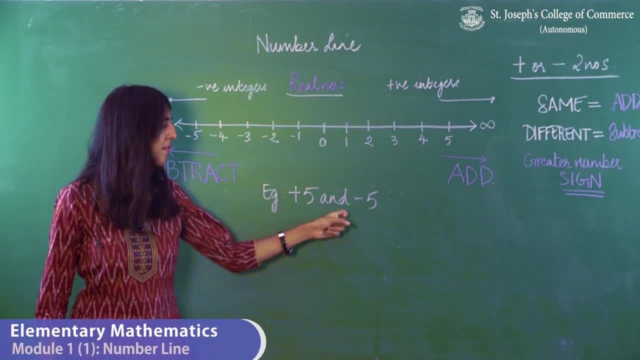 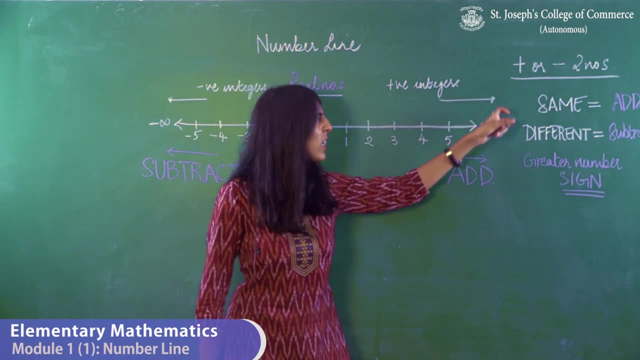 number line, two numbers are given. For example, this says plus 5 and minus 5.. Before understanding how to solve it on the number line, let's try to figure out the two rules. The first rule is that both the numbers have the same sign. you must add: If both the numbers have the 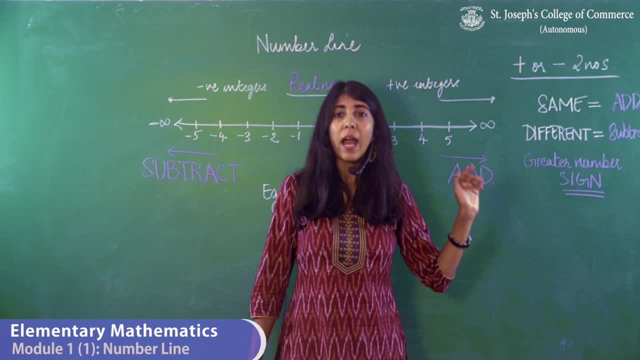 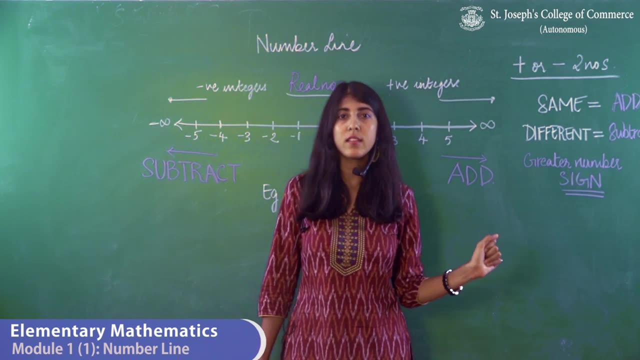 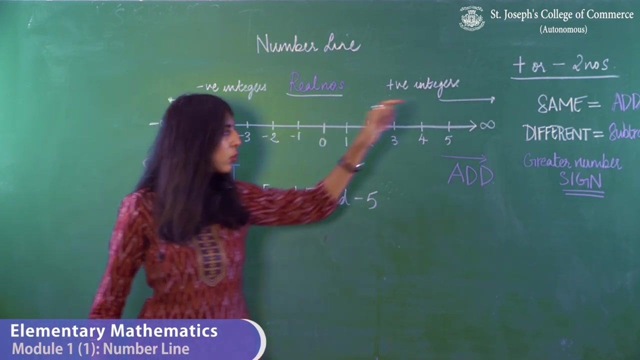 opposite or different signs, you need to subtract and then, once you subtract or add the respective numbers, the number, the answer, or the numbers with the greater sign, it's the answer that precedes it. So now, for example, plus 5 and minus 5, since they have opposite signs, you 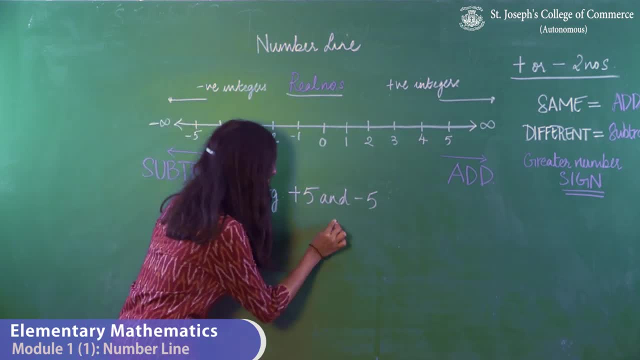 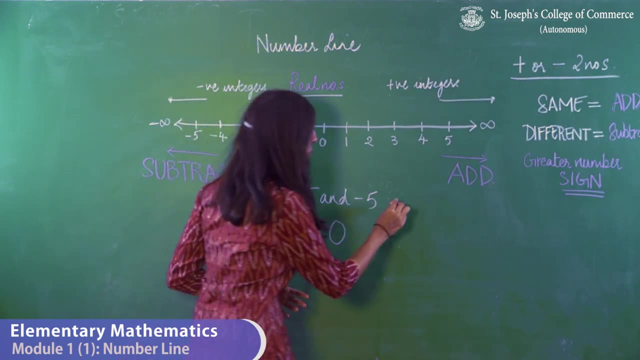 need to subtract. according to the rule, When I subtract 5 and 5, I get a 0.. In this case, 0 cannot have a sign, a positive or a negative sign, preceding it. For example, if it is minus 3, then it is 0.. If it is minus 3, then it is minus 2.. If it is minus 3, then it is minus. 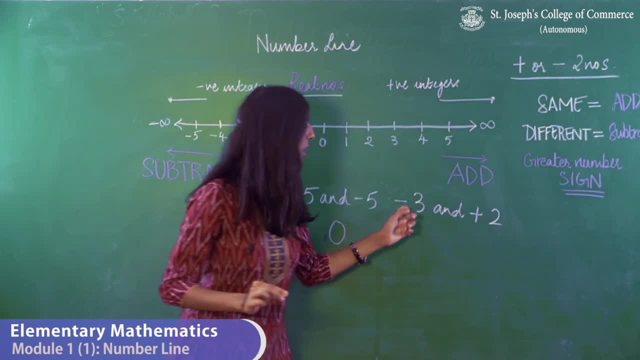 2. If it is minus 3, then it is minus 3.. If it is minus 4, then it is minus 3.. If it is minus 3, then it is plus 3, then it is plus 2.. It has the opposite signs, so I subtract. 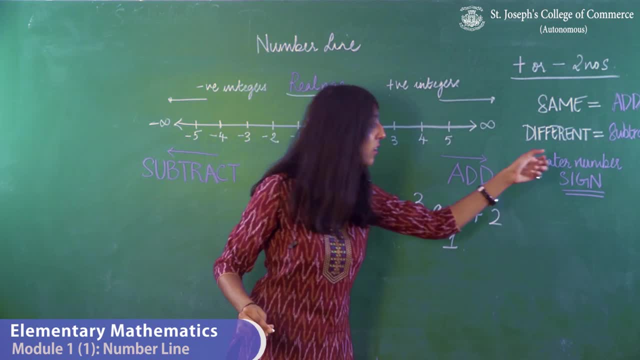 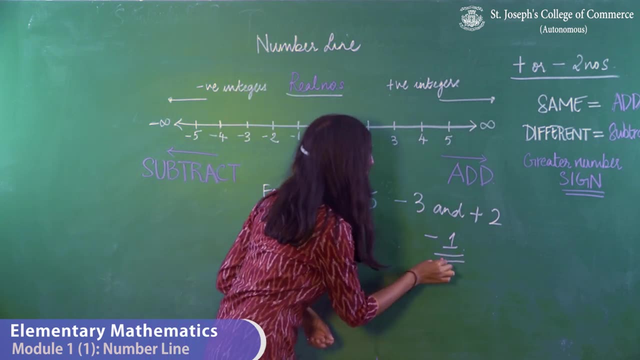 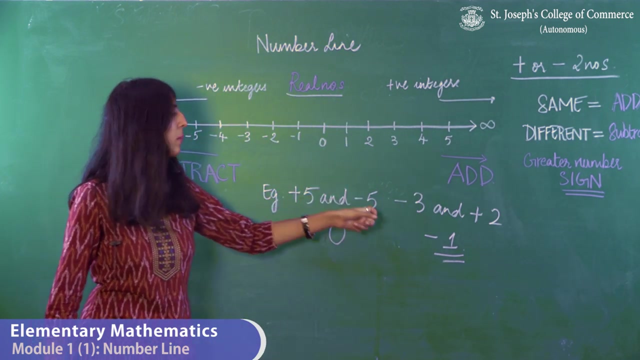 When I subtract 3 and 2, I get 1.. The greater number is 3.. The sign preceding the greater number is minus. therefore, the answer also has minus. Now let's try to understand how you solve it on the number line. Let's start with plus 5 and minus 5.. Now, plus 5 I need. 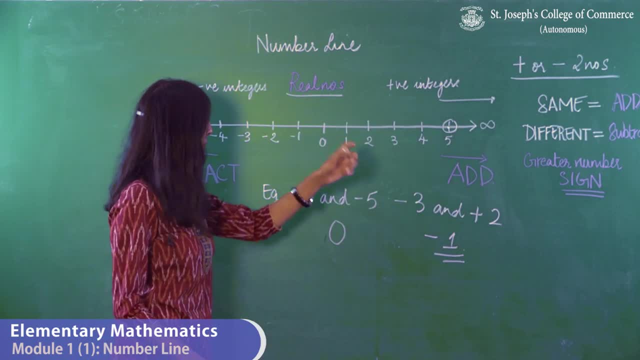 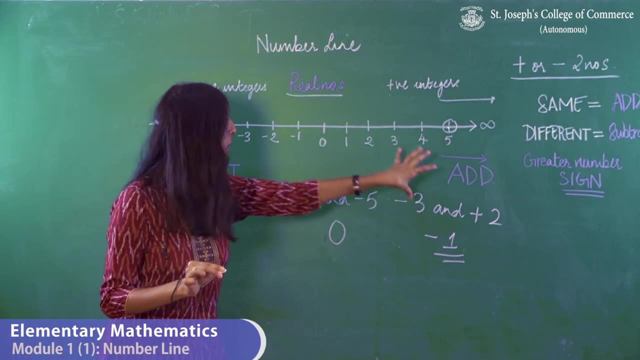 to plot it on the graph on the number line. sorry, Minus 5 is over here. As I said, when you're moving from one place to another, you need to understand what to do. So plus 5 is over here. they've asked. 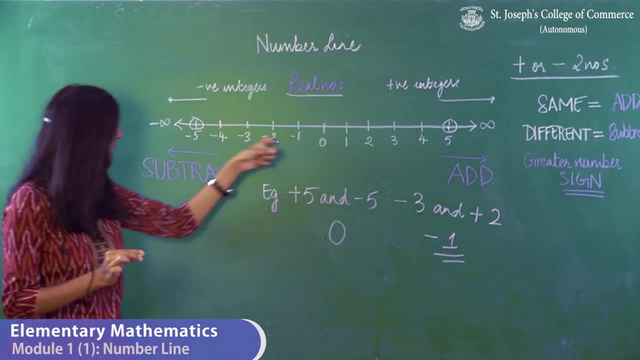 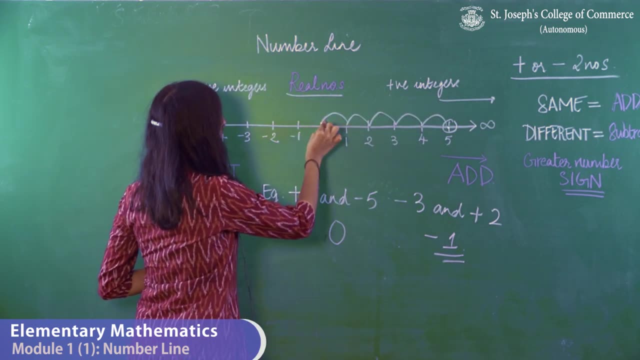 you that it is minus 5? the next number I said: when you're moving left on the number line you need to subtract. So I move 5 spaces left. So I go 1,, 2,, 3,, 4 and 5 and this is. 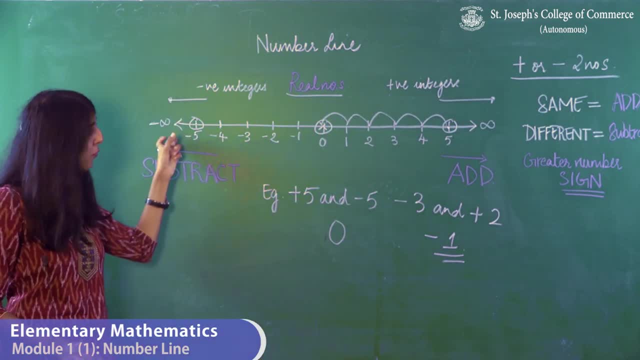 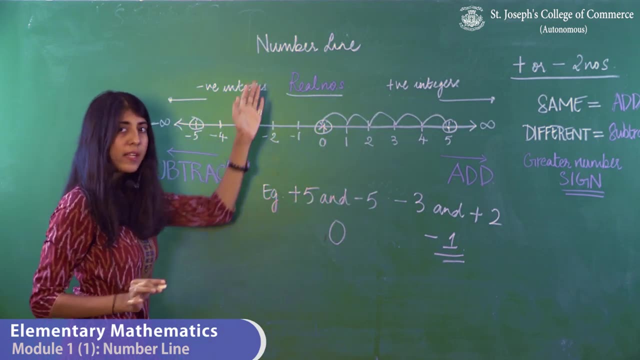 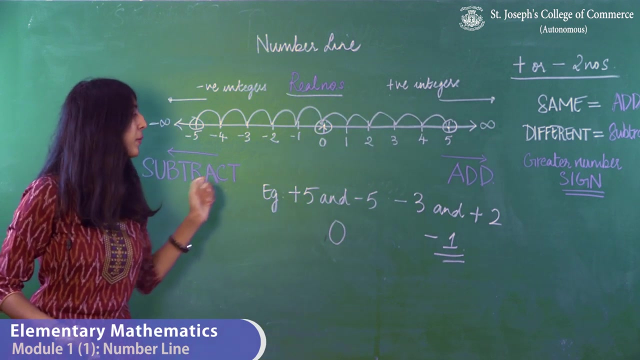 where you end the answer. Now, if I move from this side and start from here, so I say minus 5 and the next thing says plus 5.. When I have to add I need to move right hand side on the number line. So I move right 1,, 2,, 3,, 4, 5. You get the same answer, irrespective. 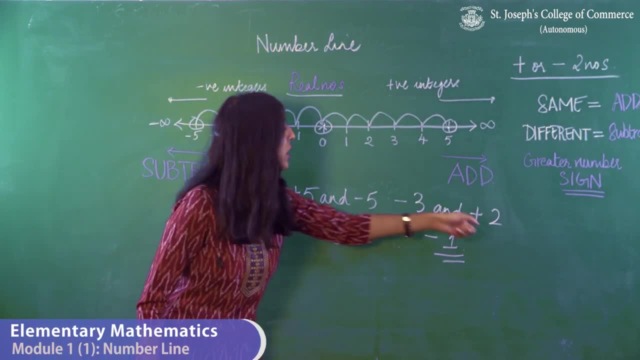 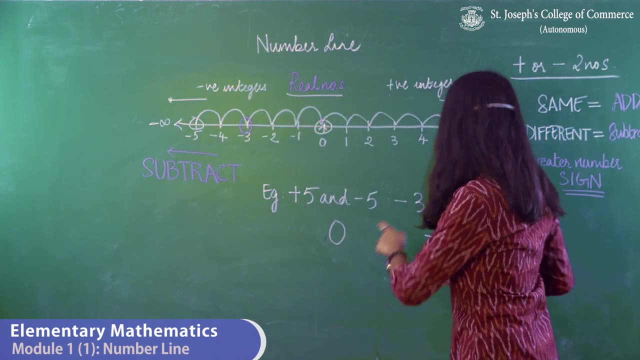 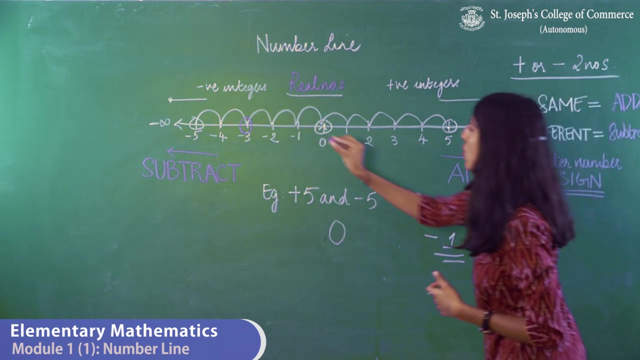 of which number you start with. Let's try solving minus 3 and plus 2.. Minus 3 is over here. okay, Minus 3 and plus 2.. If I say it's plus 2, I need to go towards the right hand side, because it says add So. 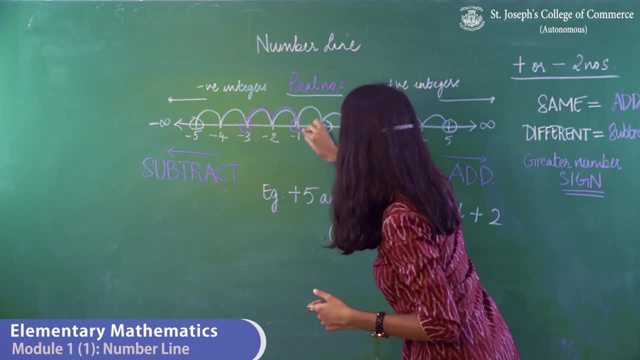 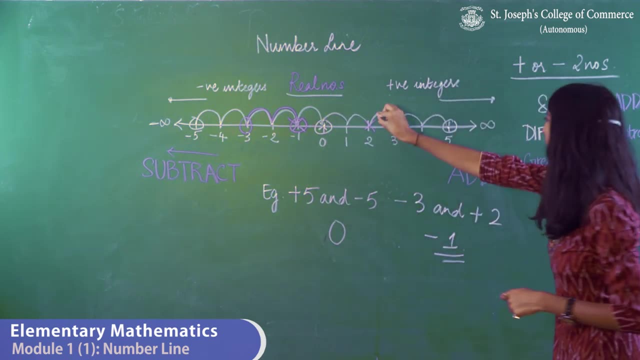 when I go 2 spaces right, I end up at minus 1, which is the answer. Now, if I start with plus 2, let's say, for example, I start with plus 2.. Plus 2, it says minus 3.. That means: 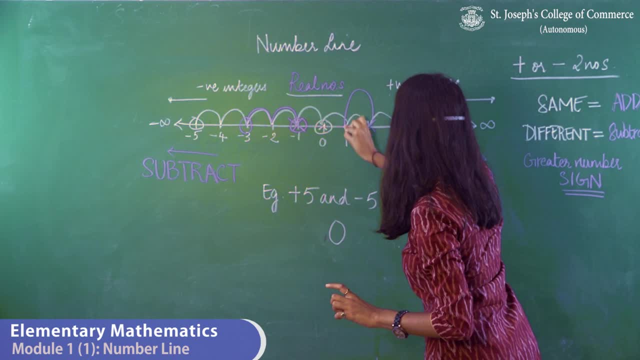 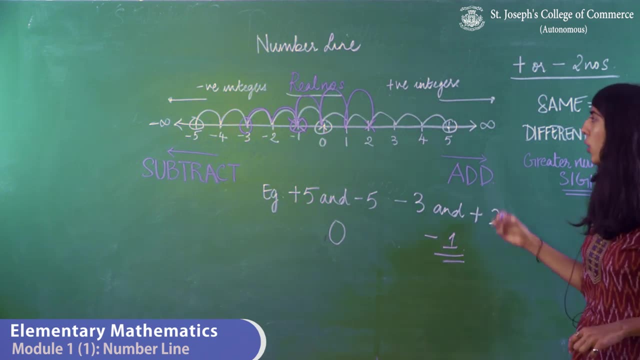 I need to subtract 3 spaces on the number line. So I go 1,, 2 and 3. I still end up at minus 1.. So whichever number you start with on the number line, you'll end up at the same answer. We just need to understand that. if I have to,